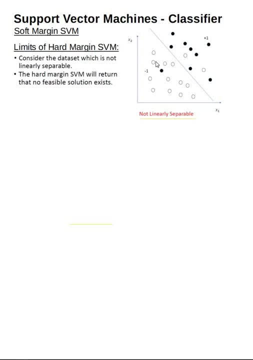 the dark circles and the minus 1, which is the empty circles. We have had a dark circle move over into the space of the minus 1, which is with the empty circles, And the same way we have multiple empty circles moved into the space with the dark circles, And this is how things are going. 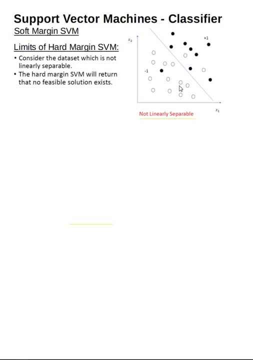 to be in practice, where linear separation is not always feasible. So in such a case the Hard Margin SVM fails to give us a solution. And what gets to happen with the Dual Formulation which we derived on Hard Margin SVM is the alphas will start converging to infinity. 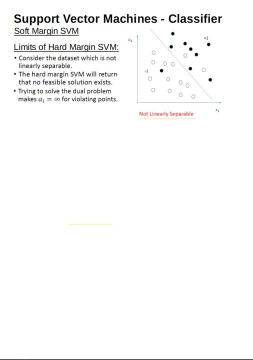 And that is a problem. so, therefore, we have now to come up with an idea to resolve this problem, And lets look at that idea, and also the formulations for that idea, as we go along. The first thing we're going to do is we are going to allow the errors to stay in our optimization. 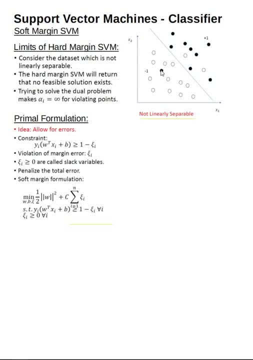 So what that means is the errors in this particular context. if the errors are there, then let that error stay, but we will actually compute a cost for those errors. so in this particular case, the difference between where that error is, in this case the dark circle, is in this side with respect to the margin. 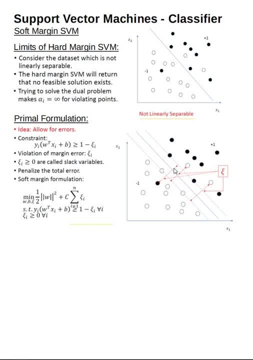 space where it is supposed to be constrained. that difference is being called the psi. so this psi symbol is indicating to us the violation of the margin. okay, so, instead of these data points to be constrained within their own margin, now they violated it and that difference is going to be. 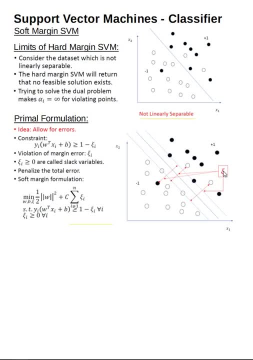 the violation of the margin. okay, and for the values that are greater than zero. so psi is only greater than zero for all the data points where there is a violation of the margin, which means the dark circles came over to the side, and then the values that are greater than zero. so the values that are. 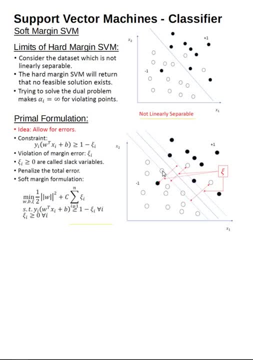 greater than zero. so psi is the same as the other values, but the data points that are greater than zero are actually the same. but that is not the case with the dark circle, because they are not the same. and then the dark circles came over to the side, which it was not expected to be, and then the 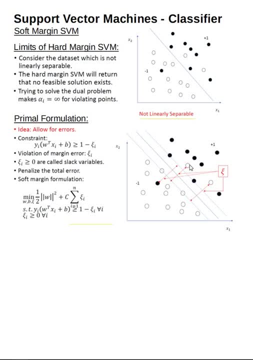 circle, empty circles have gone over to the other side, which, again, they were not expected to be. so these are these data points and these I are also called slack variables. okay, and now what we are going to do as part of our optimization is we are going to make small adjustments in the optimization. 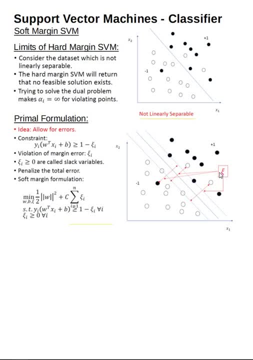 to penalize for the given psi values. so the first thing we are going to do is we are going to be updating the containing values for the given values. so we are going to update the containing values that we had earlier, which is: this is very similar to last time, where we have 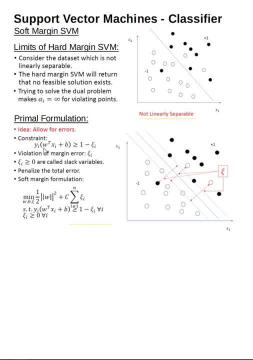 had a Y I into W. transpose X I plus B greater than equal to 1. now we have had an extra term here where we are separating the total errors or the given error contributed because of the violation of the margin. so that's a first change we make into the constraint. okay, the second change we are going to: 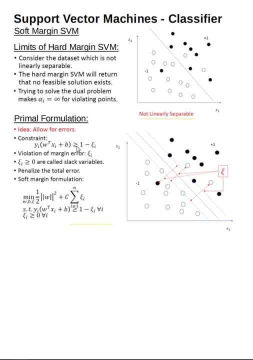 be making is to the objective function. so what we want to do is we want to penalize the objective function for any of the violations of the margin. therefore we are going to add that back into the minimization objective function. minimize of half W num, the whole square plus C, is our hyper parameter and for 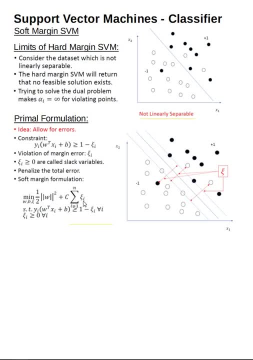 this hyper parameter. we are multiplying it with the sum of psi values, which is the sum of all violations of the margin of the particular margin. okay, so this is the new primal formulation that we have come up with, that we will try and optimize the solution for now having 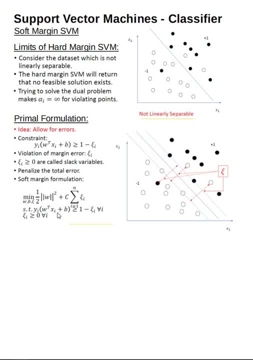 talked about primal formulation. we also are interested in finding the dual formulation and there is a very strong reason why we are doing dual formulation in the last two series, which you will start understanding when we do kernels. but right now we are going to be looking at the dual formulation and obviously 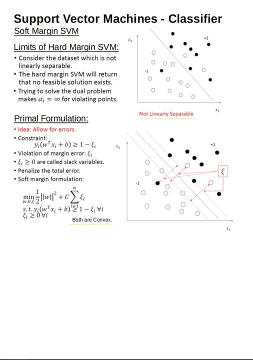 the first assumption that underlines the dual formulation is that the primal formulation is firstly convex. therefore, we can use the convex theory, which gives us the theorem that the results of both the primal and the dual formulations are the same if it is a convex problem. ok, so now moving on, let's look at the dual formulation. so, dual formulation on. 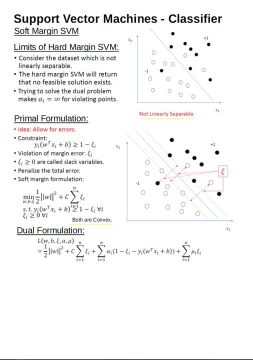 a lagrangian basis is very similar to the dual formulation lagrangian that we saw in our previous hard margin SVM, where we have half W norm, the whole square plus. this is the new term where we have added in the penalty C, which is a hyper parameter for the sum of psi i's plus. 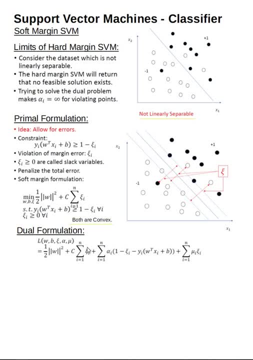 this is very similar or is the same as the one we had in our hard margin SVM, which is the sum of alpha i's into 1 minus psi i. this 1 minus psi i is coming because we change the constraint. earlier it was 1 minus yi times W. transpose X i plus b, now it is 1 minus. 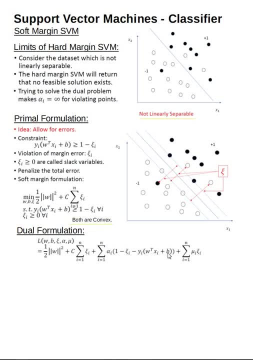 psi i minus yi times W transpose X plus b. so this is one of those. terms have gotten changed and also we have an additional term which is the mu i psi i. ok, so this is the lagrangian we have written down, where we definitely do know. 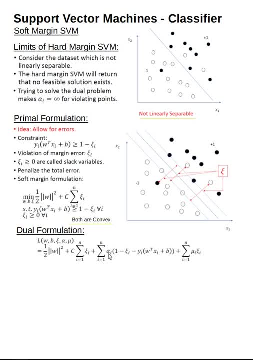 the lagrangian penalty term is the alpha. yeah, and then the parameter, hyper parameter for us to penalize for the margin violations is the C and psi i is indicating and that the extent to which a particular data point is violating the margin. ok, all right. now, very important to note: the higher value of C penalize this. 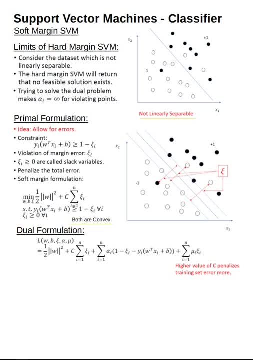 trading set more and more and constrains it to a space to ensure the size are limited. so that's very important to know now. when we take a differentiation of you know we take derivatives for this particular lag range and then we simplify what we end up with with this particular formula. 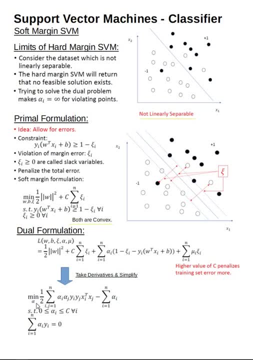 which is again a minimization problem. so what it means is we are trying to minimize over an alpha half of summation of alpha high, alpha J. i mean alpha J yiyj, X transpose I, X transpose J. So this should look similar, familiar to you from our hard motion SVM. 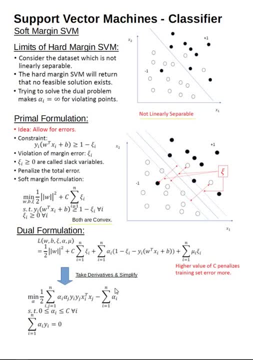 Minus the sum of alpha i's, which again is similar to our previous one, Conditional to alpha i, y, i is equal to 0. So most of this particular derivative looks very similar to what we have had And, one important thing to notice, we don't have w's here. 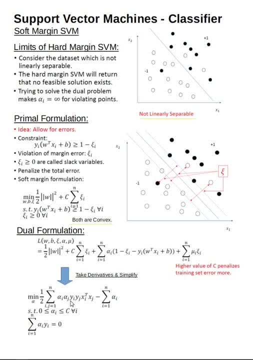 We don't have xi i's here. We don't even have b's here, which are all constraints and the parameters and values. We don't have them here. The c is brought back in here as part of boundary condition of how far this particular values should be ranging. 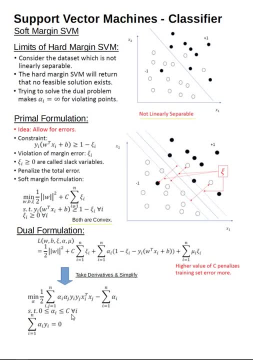 And that should be between a 0 and a c. So that's the key formulation with which we will be running a gradient descent or any other optimization algorithm for us to find the values of the parameters. Once we have alphas w and b can be calculated as w is equal to the sum of alpha i, y, i, xi. 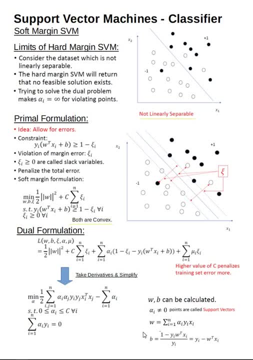 which is similar to what we saw in hard motion SVM And also b is 1 minus y i. w transpose xi by y i, which is nothing but y i minus w transpose xi, which is something in the linear regression space. This is what we typically assume as the error, where we're given the actual point. 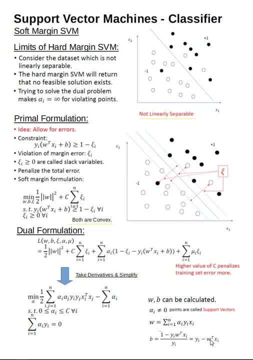 and it is the point. So the important thing to take away is the results from both the dual formulation and the primal formulations are going to be the same, And thus we have two of the formulations which we will be using in our optimization, And in our subsequent lecture we will connect all the dots of why we spend time for dual formulations. 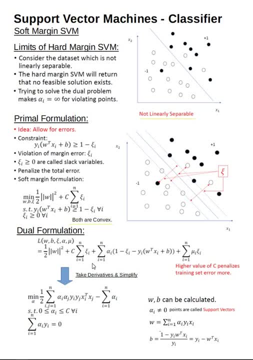 by going through the details of support vector machines, kernels and the kernel tricks. Okay, so that's all for this particular lecture. I hope you guys enjoyed the video. Good luck to you Like it if you enjoyed it. Thank you Bye.